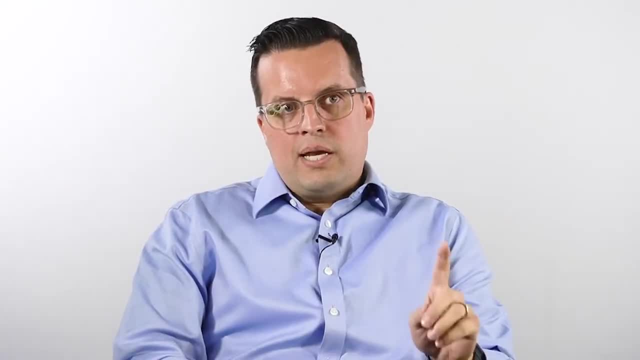 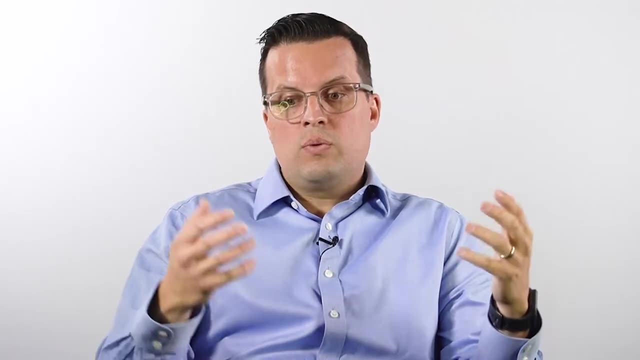 Is this a loss leader, for example? But we've got to understand what's happening with that top third of the P&L with gross margin. Is this business really worth it? And the other reason why gross margin is so important is because it pays for everything else. I like to get paid, You like to? 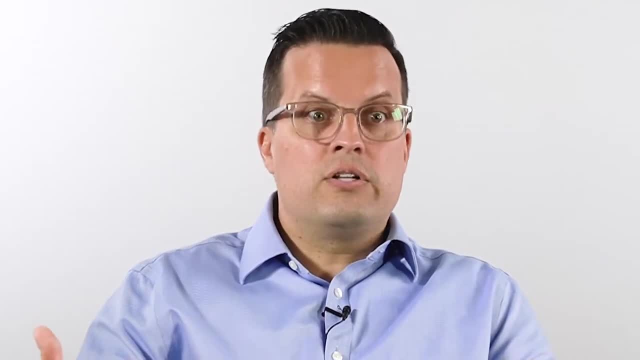 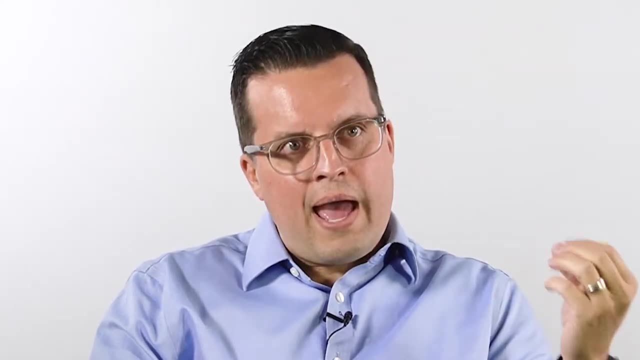 get paid. We like sales commissions, We like all of that other stuff that we get to do. We like to invest in culture and into employees And things of that nature. Well, we have to be gross margin positive, We have to be making money. 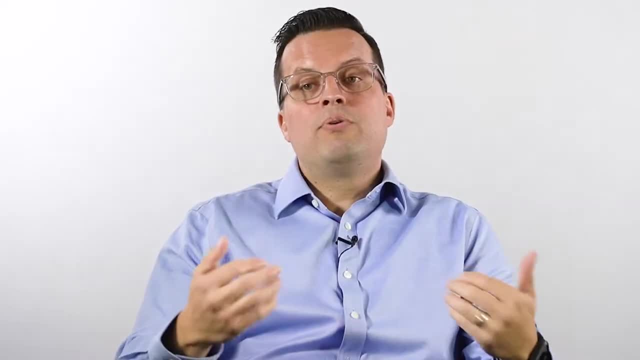 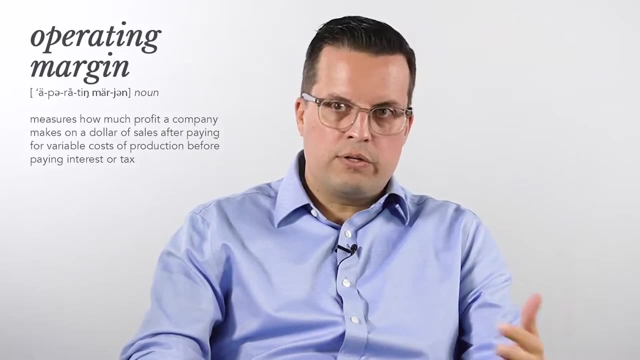 on our products and services to be able to pay for all that stuff, Which brings us to operating margin. After gross margin, we're going to subtract all of our operating expenses, our selling, general administrative expenses. Maybe we've got some research and development. That all. 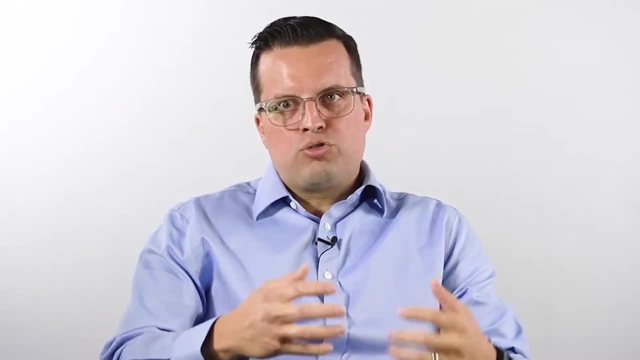 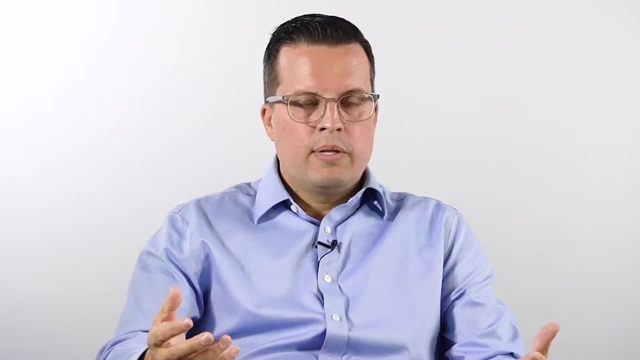 comes out of our gross margin. So we subtract those operating expenses or OPEX from our gross margin and we get what's called operating margin. So we subtract those operating expenses or OPEX from our operating income. Now operating margin is the percentage of revenue left over after we. 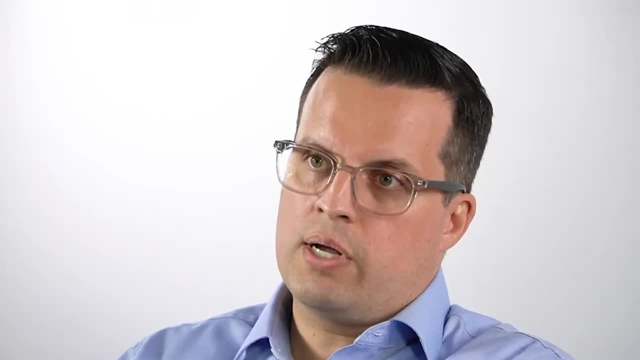 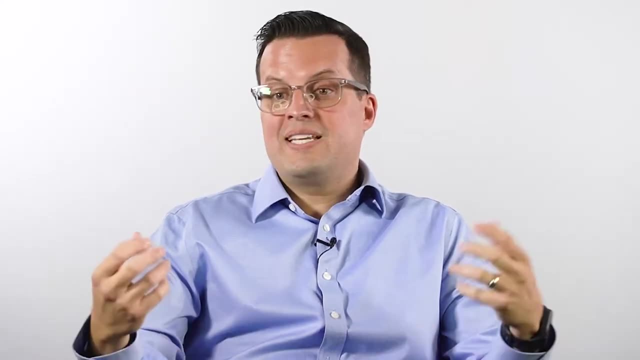 subtract not just cost of production, but also all of those support costs that we just talked about. Now, why is that important? Well, again, if we're not making money on our operations, is this really worth it? We know we're going to have some taxes. If we've got debt, we're going to have to. 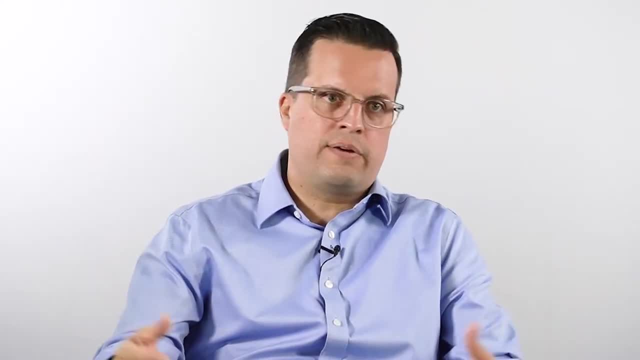 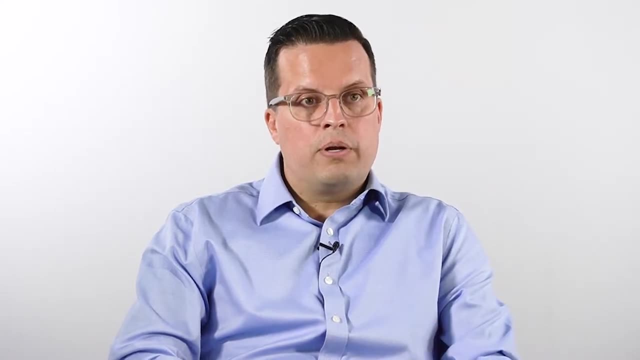 pay interest. We might also have some other non-operating stuff that we just got to take care of. So do we make money in our operations? That's what I'm going to talk about in this video. That's what our operating margin tells us. Now, when you're looking at a P&L, I think of the P&L as 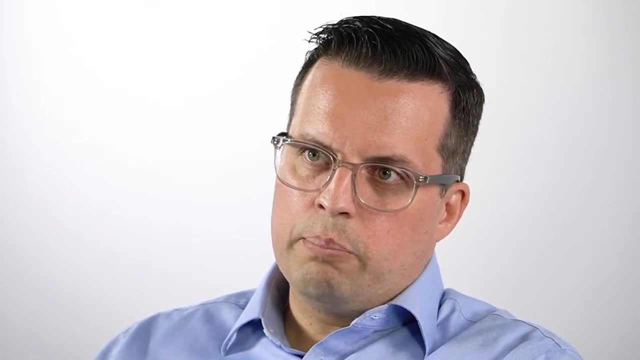 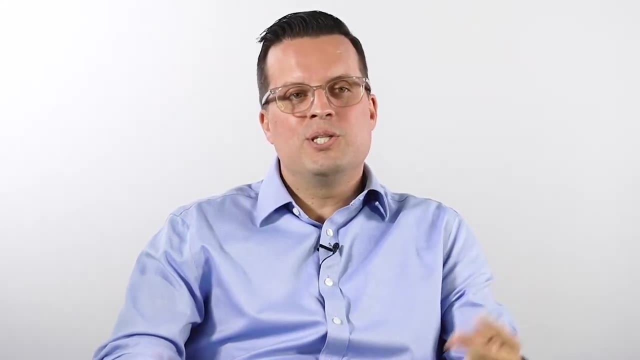 the statement of knowing what the heck we're doing, And two really, really important and really good measures of knowing whether we know what the heck we're doing is gross margin- Do we make money on our products? And operating margin- Do we make money on our core operations? So the other day, 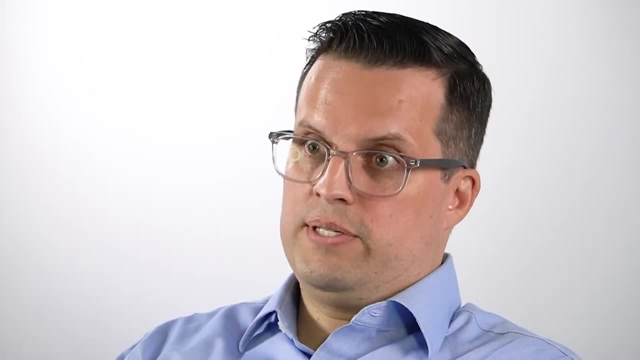 my 12-year-old son asked if he could start a shoe reselling business. He wants to buy Jordans and sell them. I said, great, let's do it. Well, he obviously needs the money. So he said, well.